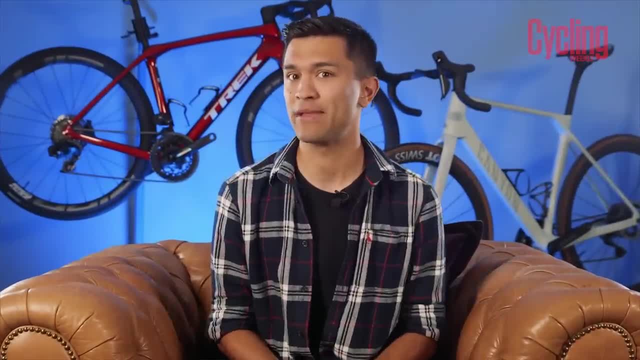 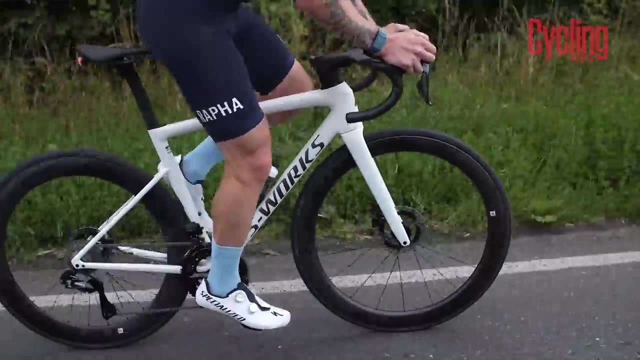 armchair critic, but being this far removed from the development process does mean that we can look at things quite objectively, And doing just that is what made me realize that there really are a few things that bike manufacturers could be doing differently. Let me explain. 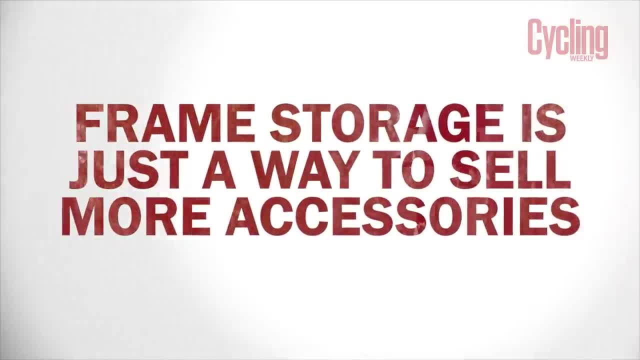 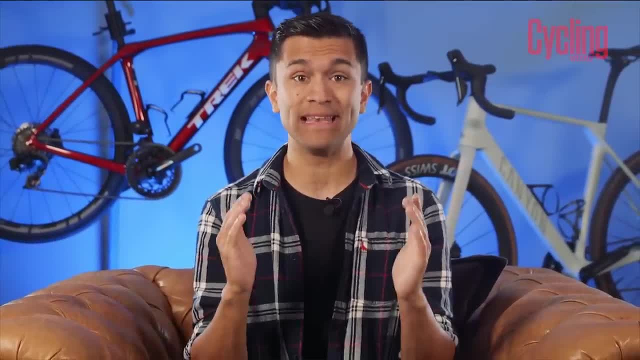 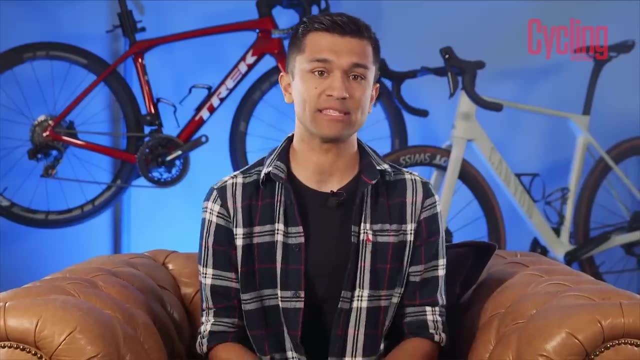 First off is the advent of frame storage, A concept that I absolutely love, The idea being is that you can utilize the space inside of your frame to store things such as tools and other spares. Multiple brands are doing this, like Specialized Trek, Orbea and, more recently. 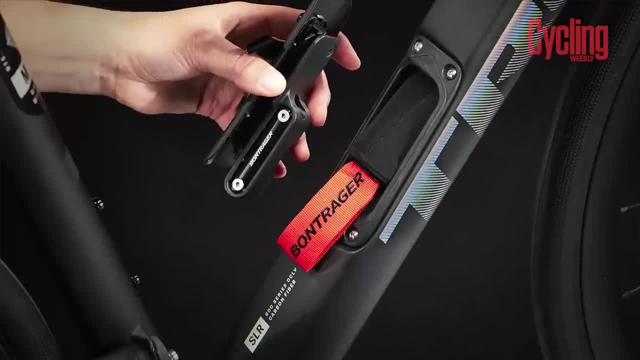 Canyon. The feature usually means that you either don't need to use a saddlebag or you just don't need as much stuff in your bike. So if you're looking for a bike that's easy to handle, you might want to start with a bike that's easy to handle. If you're looking for a bike that's, 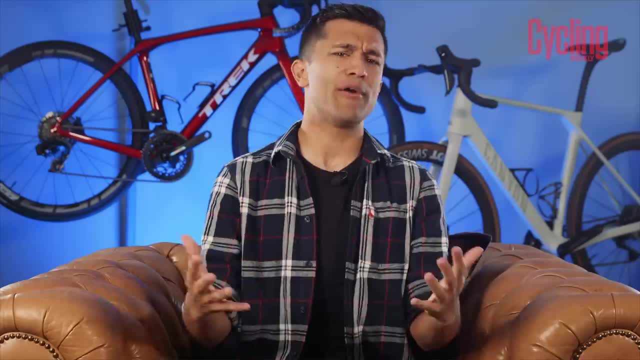 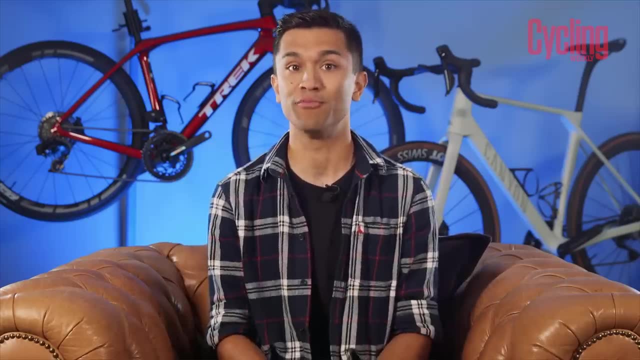 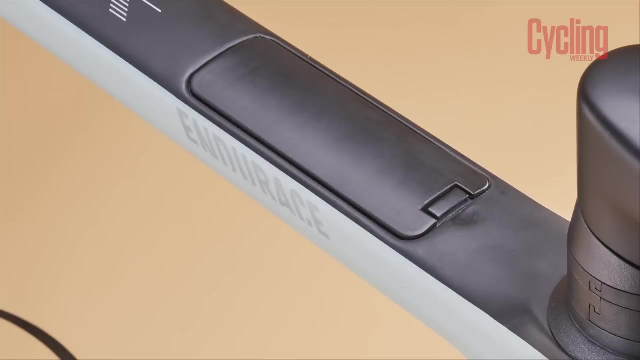 easy to handle. you might want to start with a bike that's easy to handle. However, my issue lies in the fact that even if you have spent £6,000, maybe even £10,000 on a new bike with frame storage, the manufacturers will still force you to spend a little bit more money to buy all of the 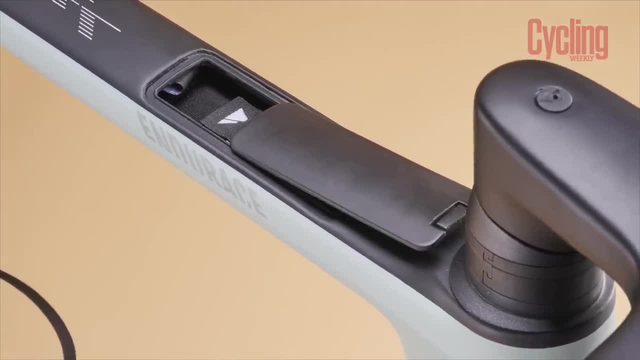 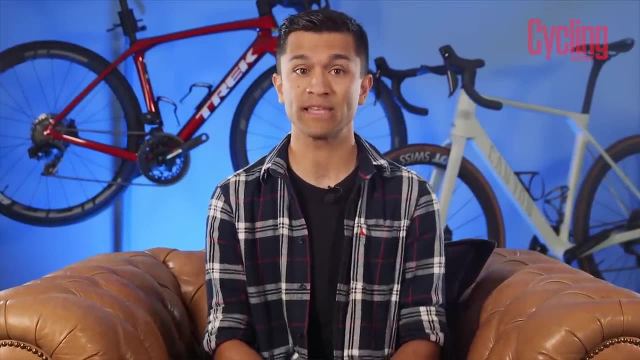 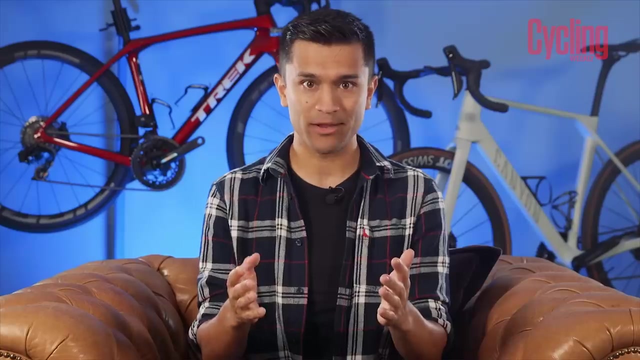 tools that were made specifically to work with its own storage solution. I'm sure there's a load of tools out there that will also fit into whatever sleeve place hosts to the tools And who knows, maybe you already happen to own those tools that will fit. But in my opinion I think if you've just 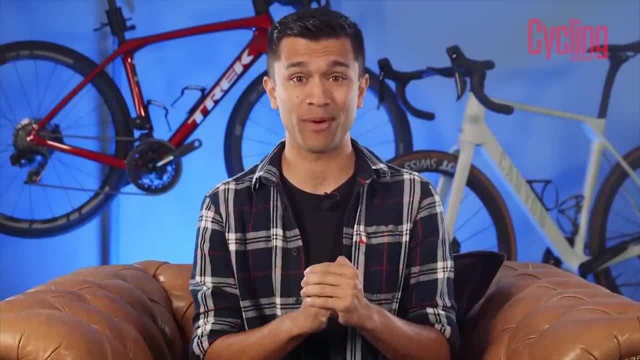 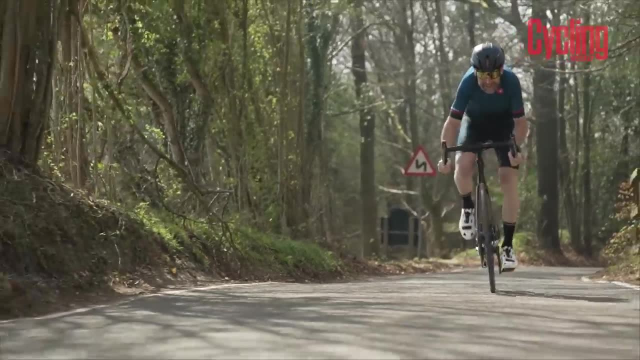 spent what is undoubtedly a small fortune on a new bike, getting the tools that go with that bike should almost just be part of the package. I also think that, since none of the brands give you a full set of accessories with your purchase, it opens up the opportunity for one. 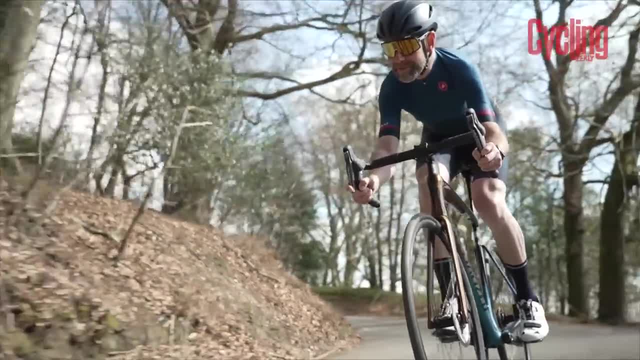 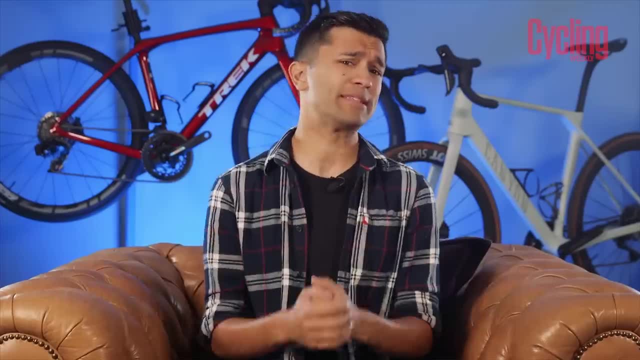 brand to rip away from the status quo and be seen to offer some exceptional value by doing so. But the question is: who's going to be brave enough to do it first? One limiting factor- a brand- I spoke about this too- pointed to the issues that surround 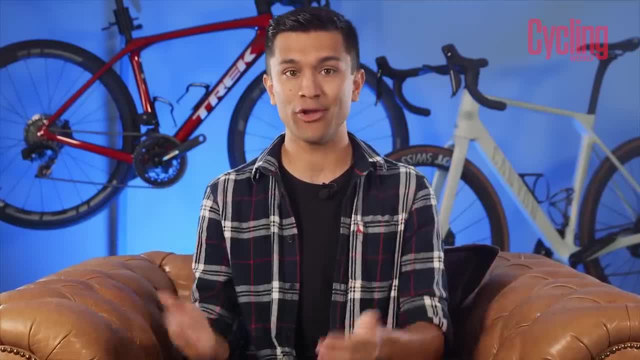 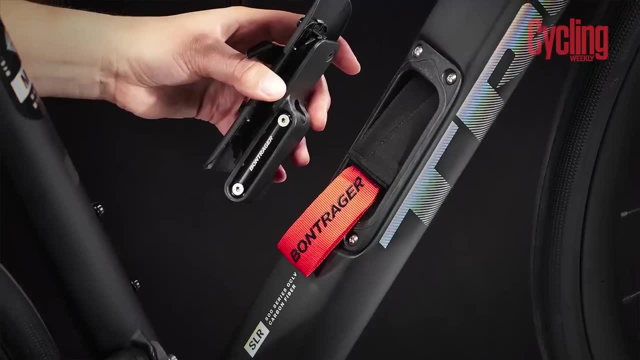 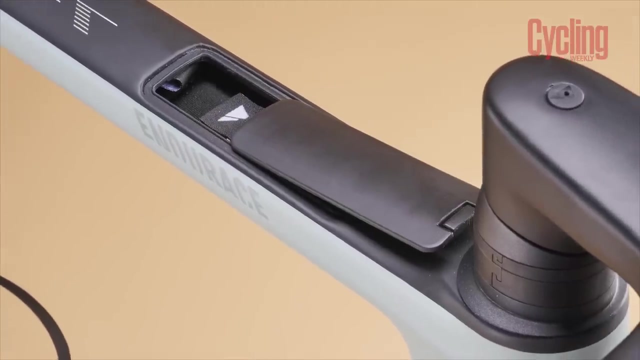 shipping CO2 canisters, which is obviously a no-go, But CO2 canisters only make up one component housed in most storage sleeves. I just don't see a good reason why the multi-tools and tyre levers have to be excluded, other than a way for them to just sell more things. 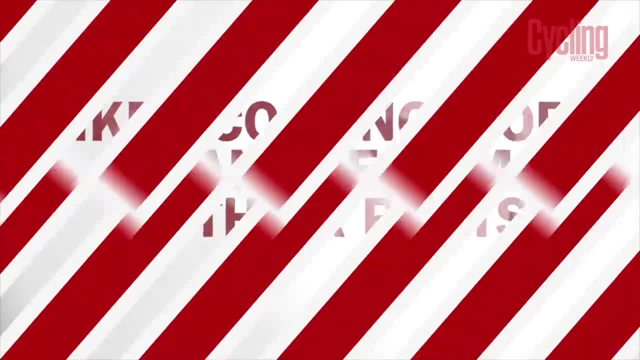 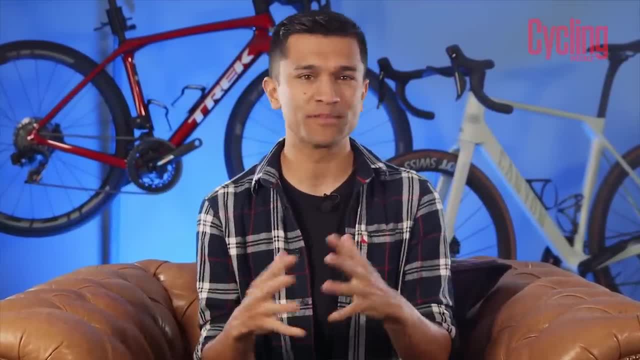 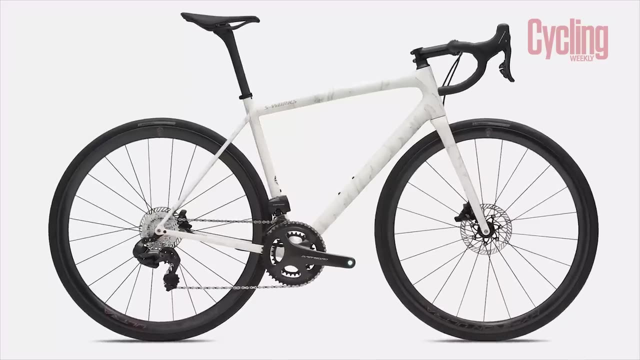 A real bugbear of mine, and it's a problem which only a few people will really care about, are bikes that cost more than the sum of their parts. The reason why only a few people will care is because the problem tends to affect bikes that sit right at the top end of the spectrum. 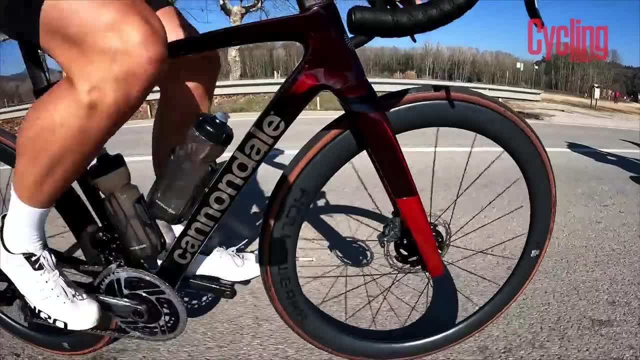 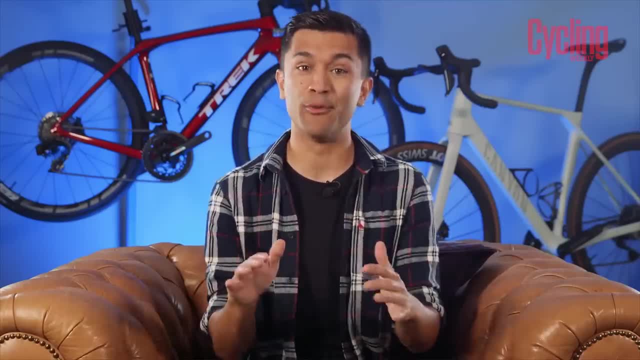 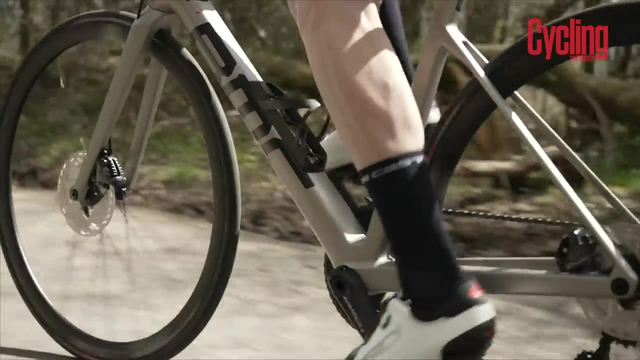 Think your Cannondale Lab 71, Super 6s, S-Works Athoses or similar. Perhaps the industry just has a problem with discounting and retailers becoming ever more ruthless with their race to the bottom on sale prices, But what it is creating is a retail environment which lends itself more to individuals. 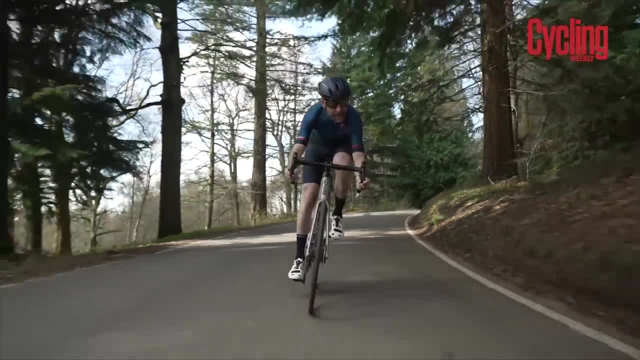 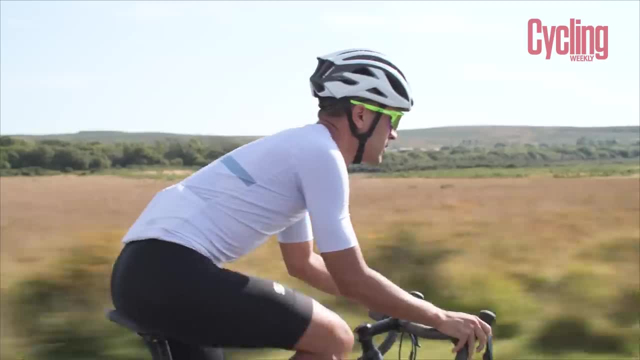 building up their own frames rather than buying full builds. Personally, this is my favourite way to buy a new bike, but for the average cyclist on the street, I don't think that they should be paying a premium just for buying a fully built bike. 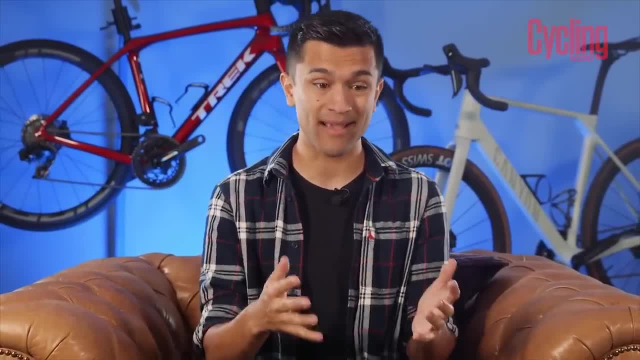 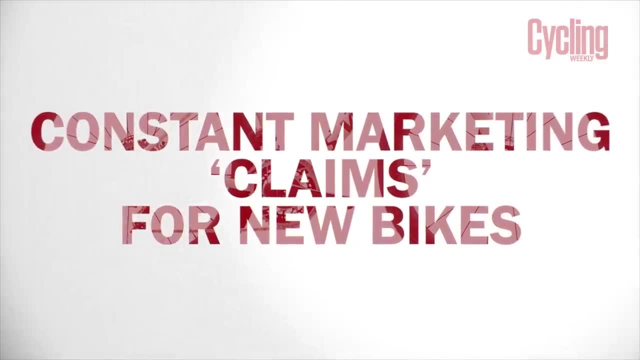 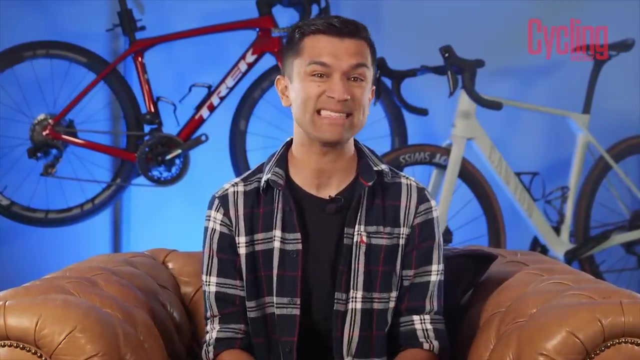 If anything, there's a strong argument for custom bikes to be the thing that cost a bit more money. New Bike Bingo: When a new bike is launched, I love playing a game of new bike bingo. We're all but guaranteed to hear about the latest offerings. weight savings. 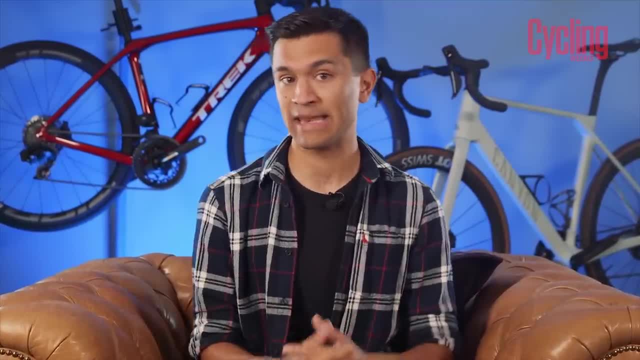 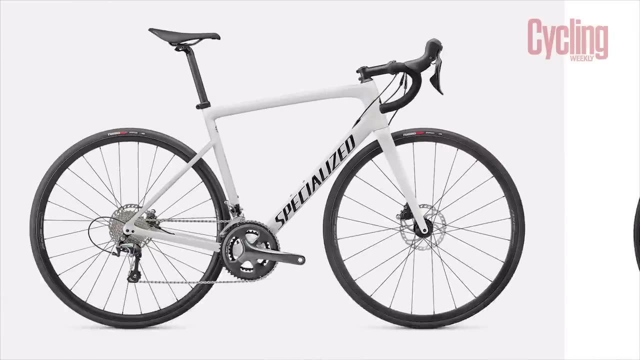 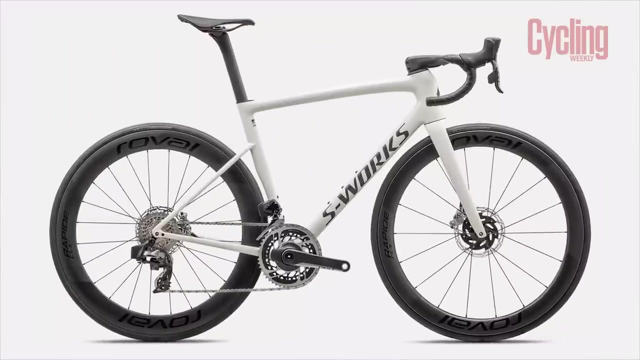 stiffness and compliance improvements, along with aerodynamic gains. While I do believe that, over the years and from model to model, bikes have been improving the riding experience for the majority of riders, the ever-present trust-us approach to new bike marketing is slightly annoying. In reality, we, as the consumers, 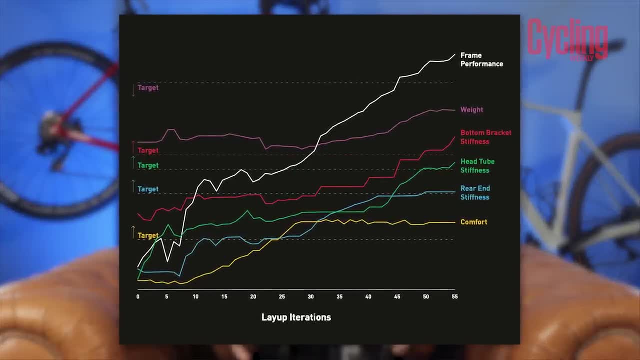 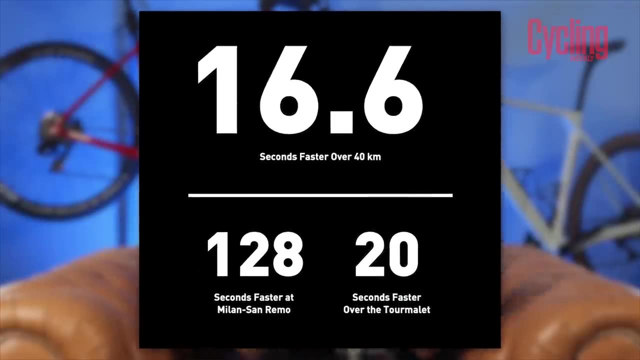 just don't have the ability to fact-check all of these numbers that the bike manufacturers lay on us when they launch a new bike. Even if you do try and go out and do some of your own testing out on the roads, the results can be incredibly skewed depending on a multitude of external 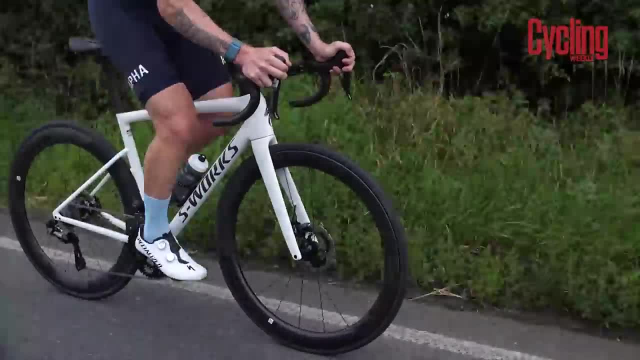 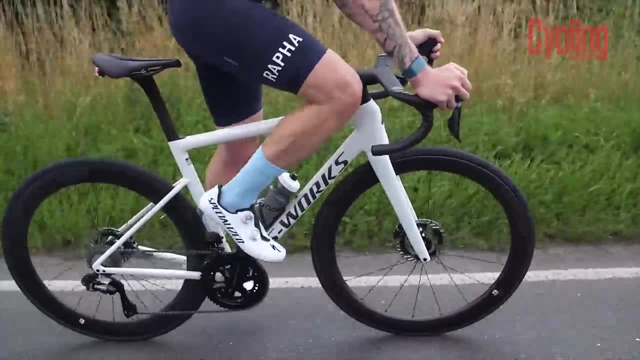 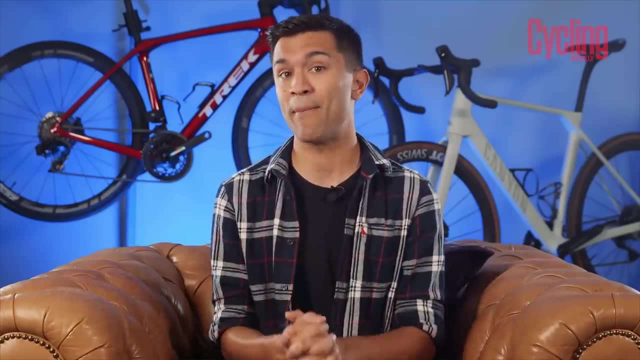 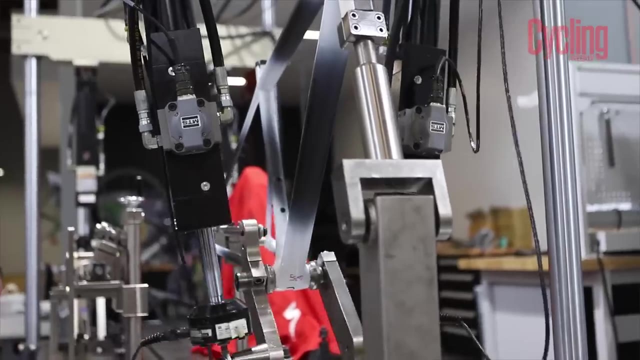 You'd need access to a pretty sophisticated rig to do so. I would love to see brands send their new bikes off to an independent testing centre to verify the claims that they're making. I believe that by doing this, the manufacturers would actually be able to gain more trust from the consumer, and it would also add 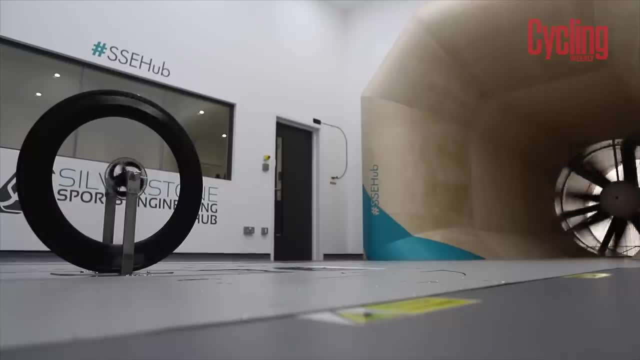 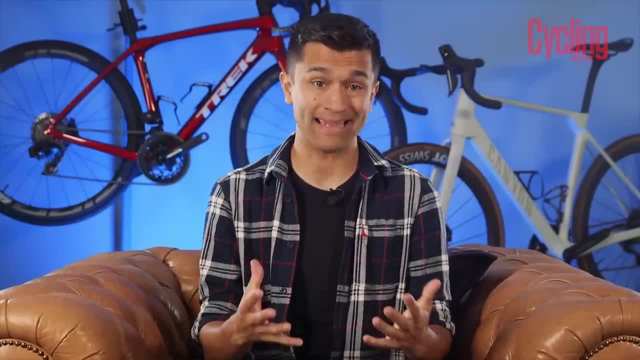 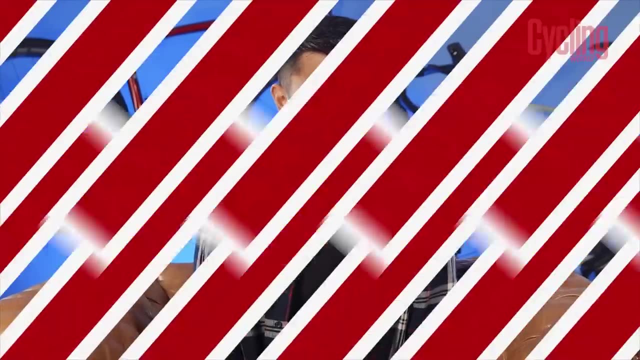 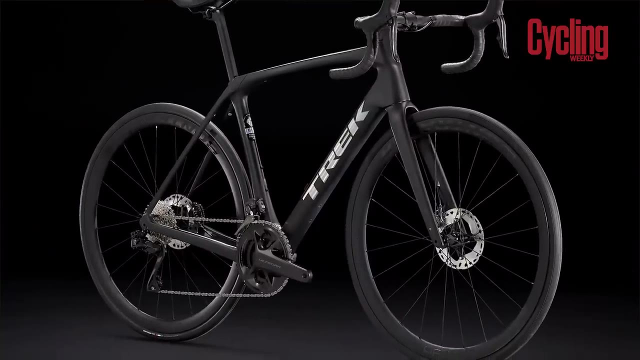 New Bike Bingo, New Bike Bingo. And tests couldn't be run that extrapolate an increase in performance which, in the real world, may not even exist. New Bike Bingo. New Bike Bingo, New Bike Bingo. When manufacturers launch new flagship bikes, the full ranges often include frameset options as well as full build models. 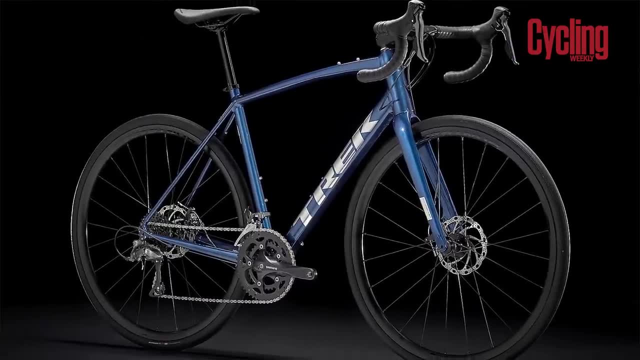 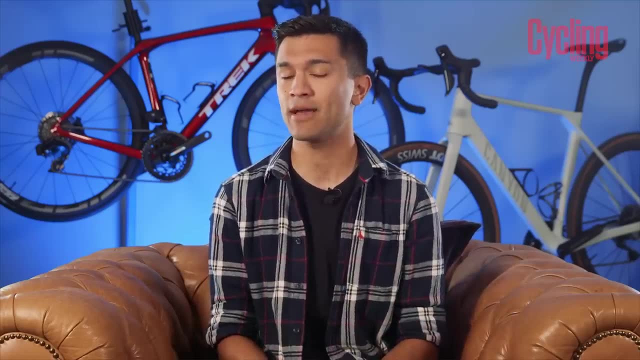 Which I think is fantastic. It's not uncommon for brands to do this, especially with models like the Tarmac SL8,, which is available in a number of different frameset colours. It provides the opportunity for customers to spec their bike however they like or if they already. 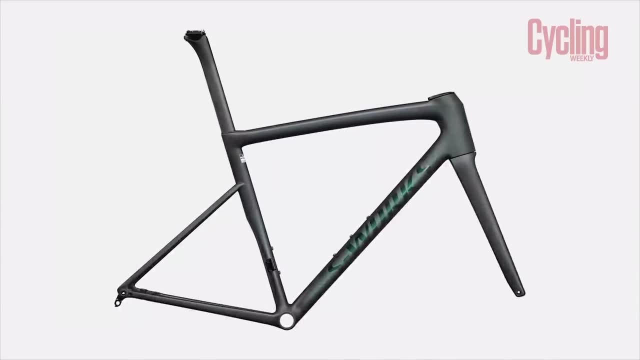 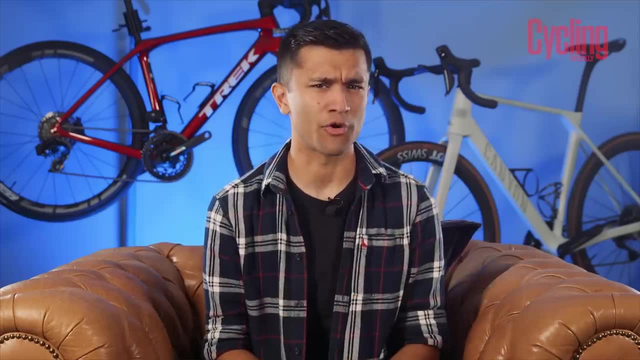 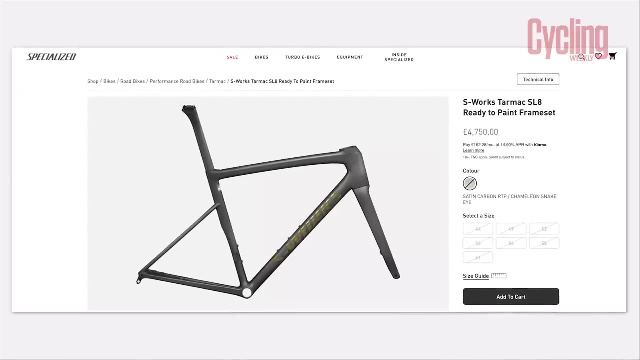 have a bike with the components that they're happy with. they can just build up the new frame with what they already own, creating a more cost-effective solution. However, one thing that isn't so common are RTP frames, or ready-to-paint frames. What these are are frames with no paint. 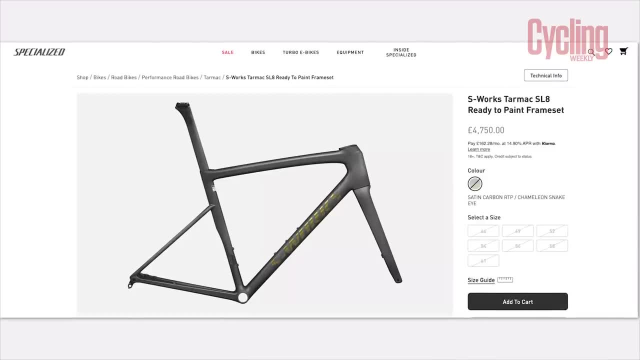 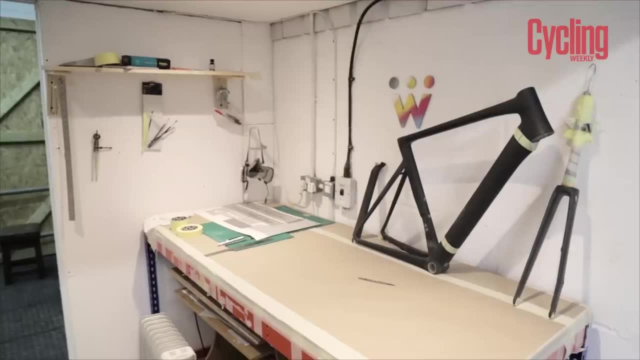 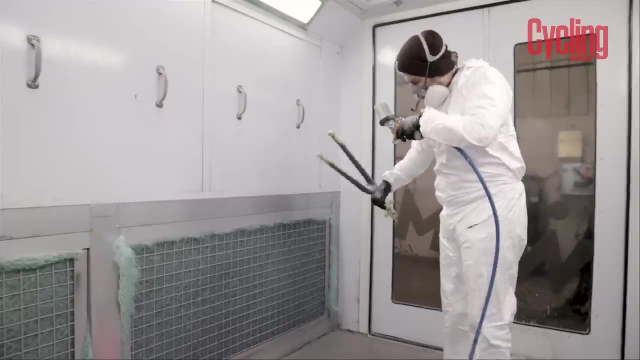 but just a very thin layer of protective lacquer. It also means that if you want to go one step further with your custom build, you can also then give it a custom paint job, and you can either save on the effort or the cost of sanding all the paint back before then. repainting The SL8 is one. 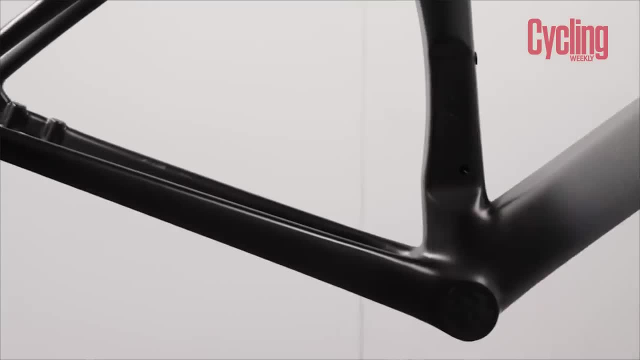 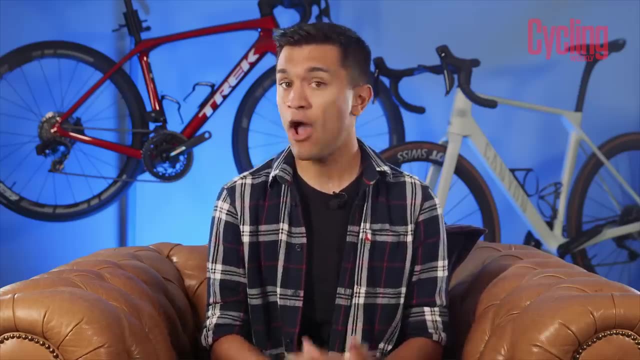 of the few framesets that is available in an RTP option. All that needs to be done is to take off the top thin layer of lacquer and the decals, and then you're good to paint. I'd love to see more brands adopt this method, but I don't think it's a good idea. 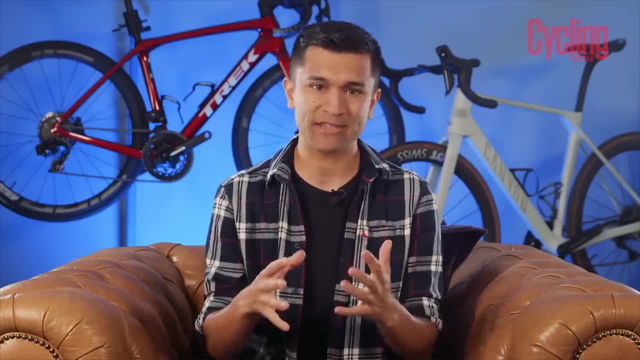 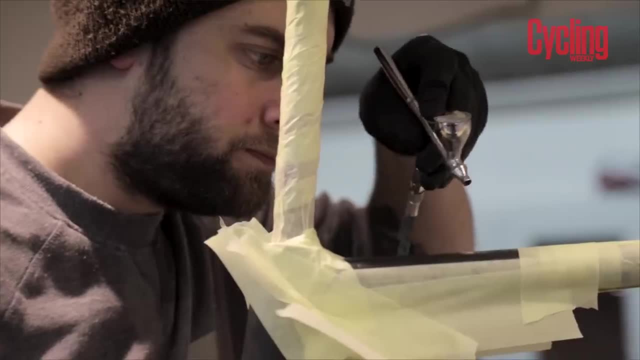 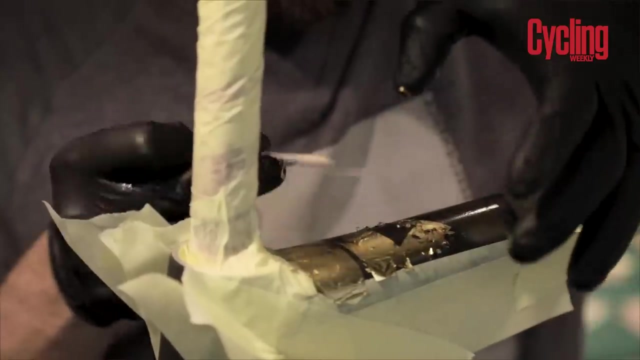 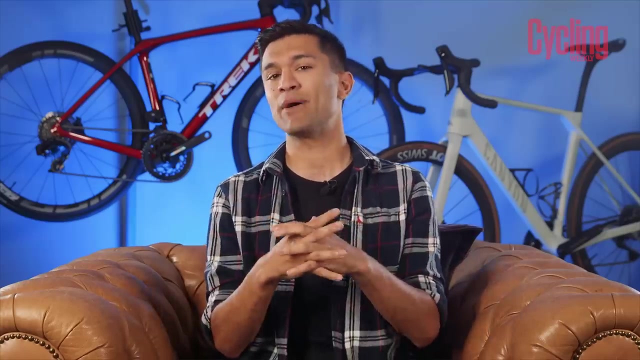 From the bike manufacturer's point of view, it negates the need for an entire step in the production process which you have to imagine, saves the brand time and money. I also believe that RTP frames allow customers to engage with the brand on a deeper level when having the option.